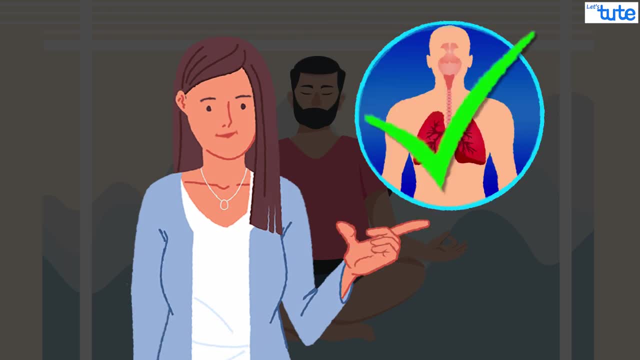 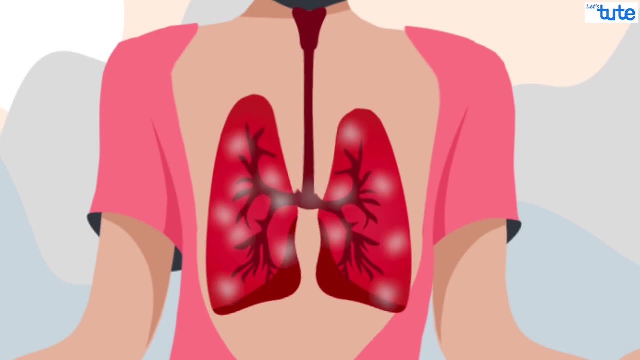 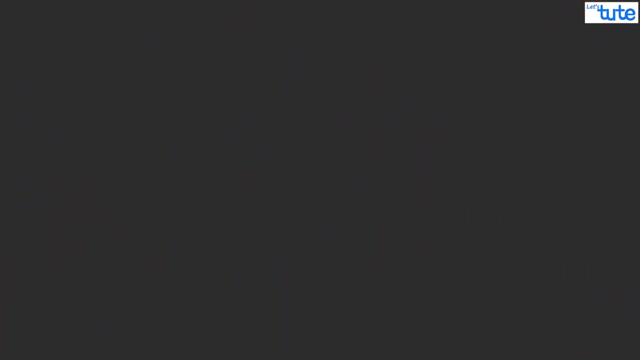 You might say it goes to our lungs. Well, yes, it is correct. The air passes through the respiratory tract and then enters the lungs. So let's explore the features and the parts of the human respiratory system. The air enters the human body through nostrils, which then passes through the nasal cavity. 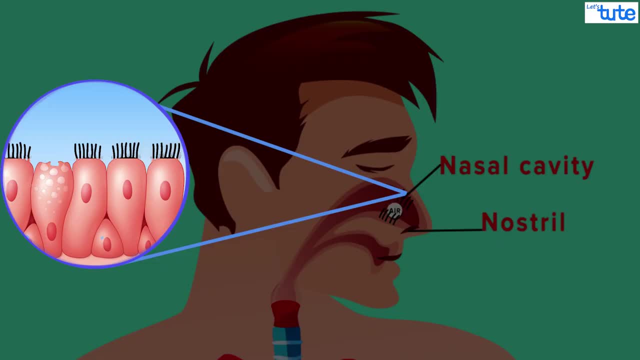 The air is filtered by a specialized hair-like structure in the nasal cavity called cilia. The cells of the nasal cavity secrete mucus, which helps to trap the dust particles and blocks it from moving ahead. The nasal cavity also provides warmth and adds moisture to the air. 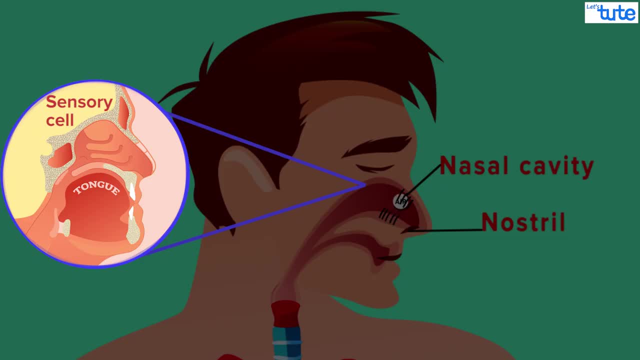 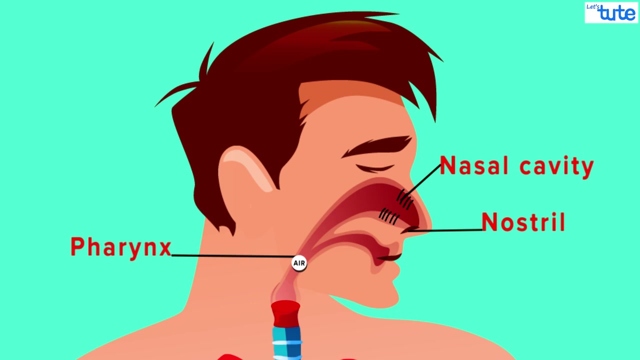 The nasal cavity has specialized sensory cells that are sensitive to smell and odor And, yes, that is the reason why our nose is a sense organ. The nasal cavity opens into a much wider cavity called the pharynx. The pharynx is a common passage for air and food. 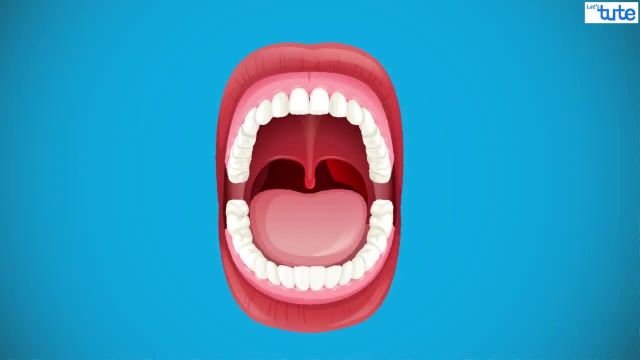 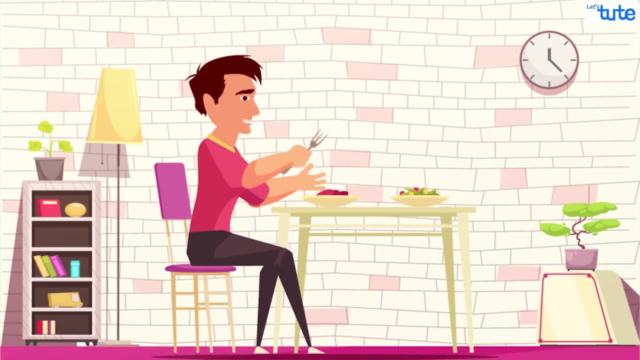 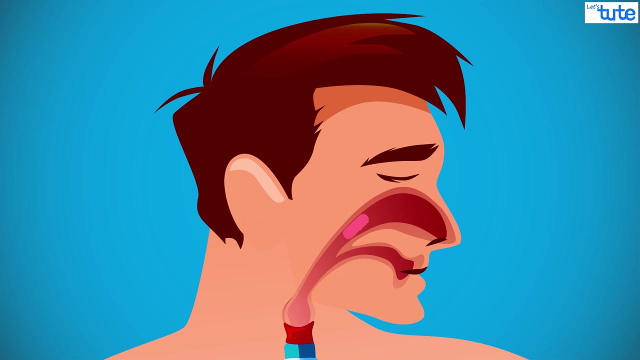 It is easily visible when you open your mouth wide. Yes, the region behind our tongue. Has this ever occurred to you that while having food, you cough because the food accidentally entered the other pipe? Well, yes, this never happens otherwise. This is because the pharynx has a cartilaginous. 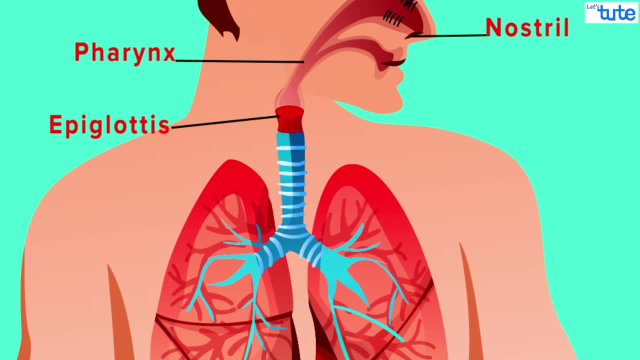 flap-like structure called a pharynx. The pharynx has a cartilaginous flap-like structure called epiglottis. This epiglottis closes the windpipe when we swallow the food. It prevents the entry of the food in the windpipe. 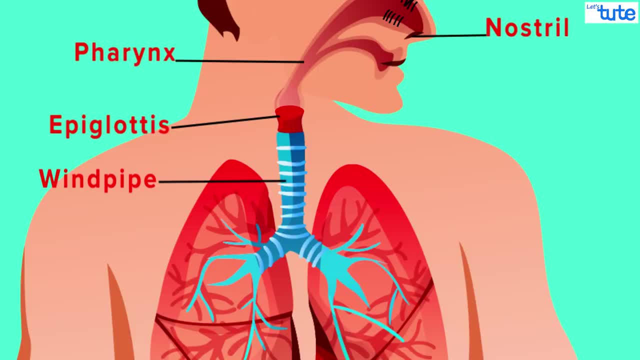 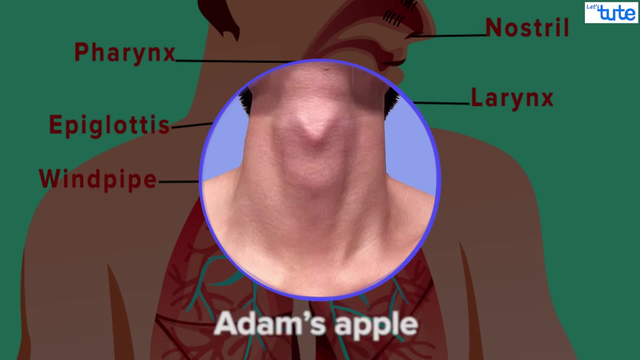 So, while swallowing, if the epiglottis is partially closed, we cough. Followed by pharynx is a region called larynx, the voice box. The larynx in males is often seen protruding out. This is called the Adam's apple. 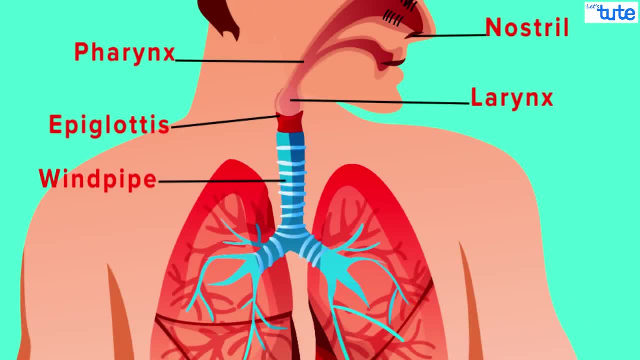 From here the air passes through a 4-inch long tube-like structure called trachea. The trachea is often referred to as the windpipe. If you carefully observe the structure, there are many C-shaped cartilaginous rings present. 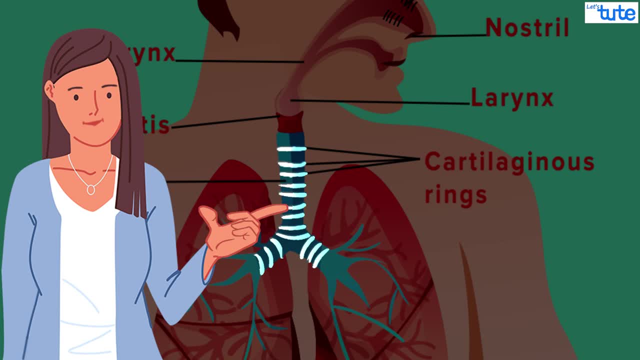 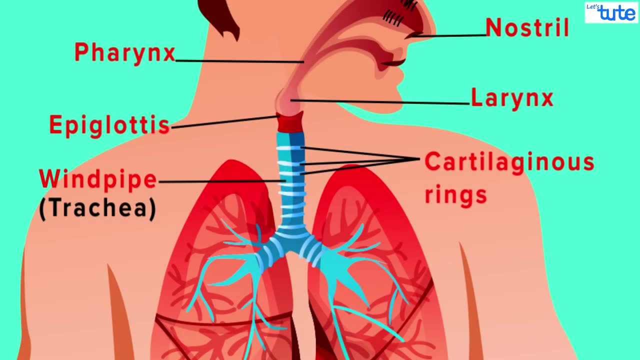 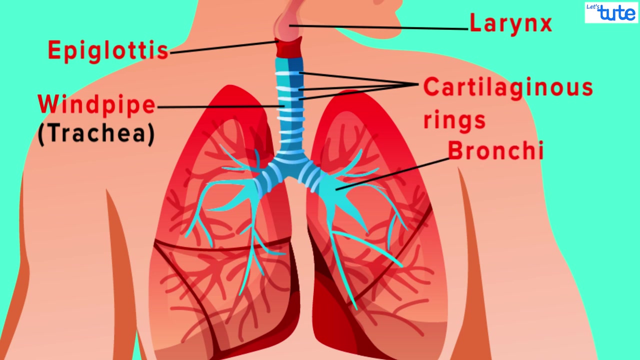 on the trachea. What do you think is the function of these rings? These rings prevent the windpipe from collapsing Close to the lungs, the trachea or the windpipe. this part is formed, or the trachea is inserted into the firstbranching tube. 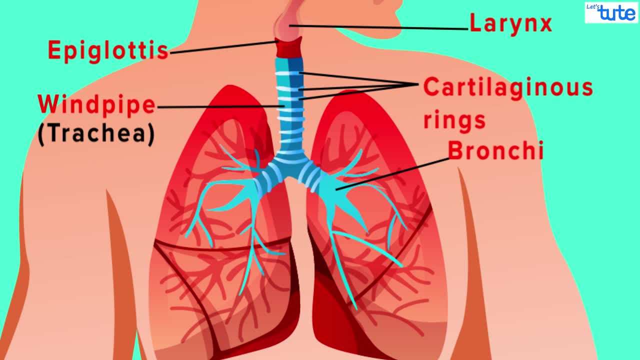 the trachea of the clavicle, The secondbranching tube starts making this 36-inch section of the trachea open. From this höfde to the diving portico and expand to the sister trachea. In both, each of these tracheas is made into. 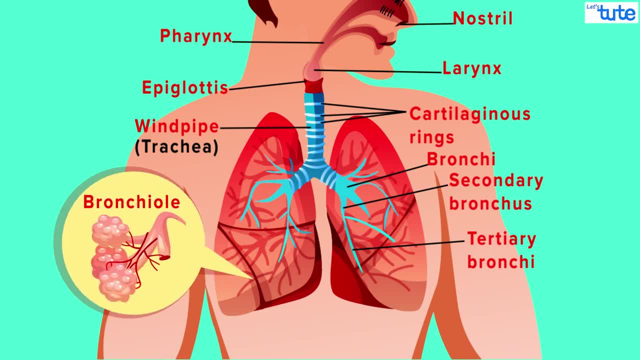 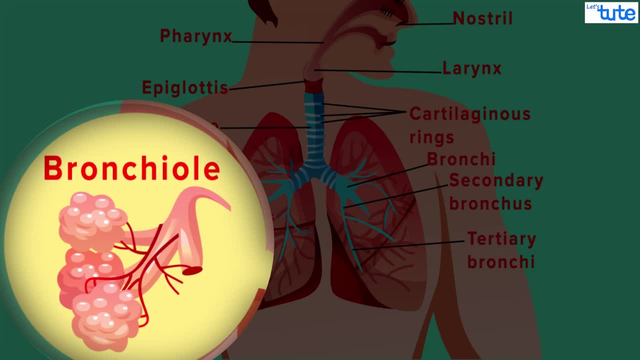 the branch as a trachea or a branch which builds up growth. Thus, if the posición is in a jointed vein, getting in and out of the joint is difficult. cluster of tiny air sac like structures called the alveoli. They are often referred to as 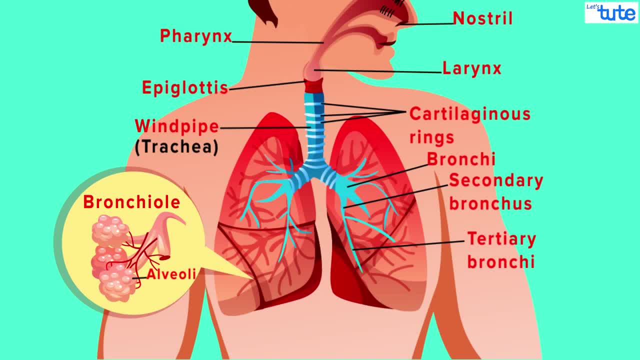 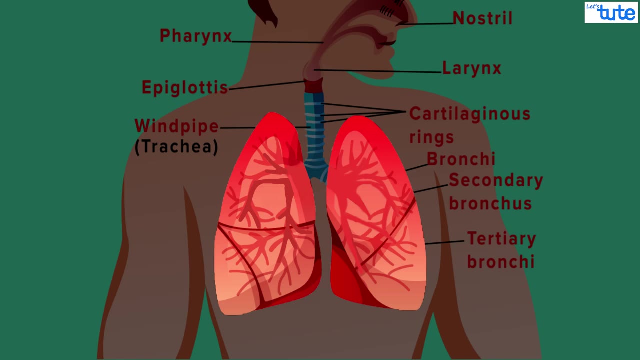 the air sacs, The alveoli are surrounded with blood vessels. They are the actual site for gaseous exchange. Now talking about the respiratory organ, lungs. Lungs are a pair of air filled spongy organs located in the chest cavity. Carefully observe the size of the lung. Are the two of the same? 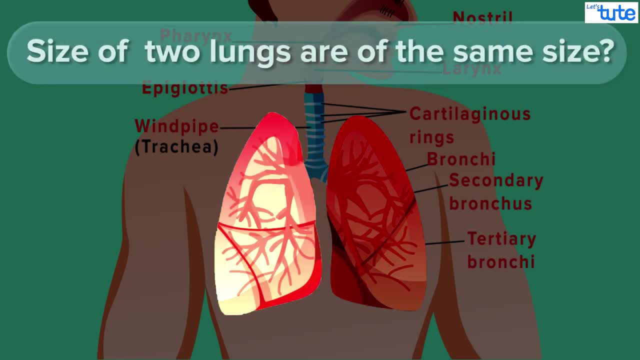 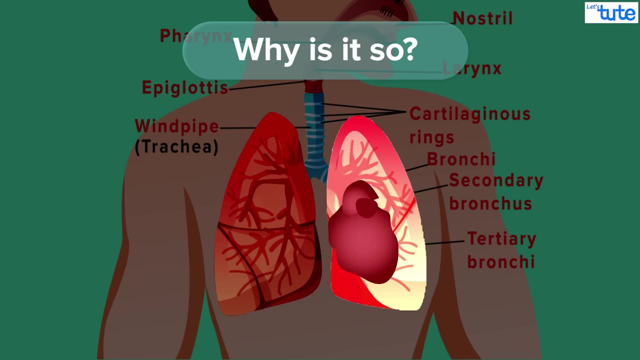 size. The right lung is larger than the left lung. Can you think? why is it so? It provides space to accommodate the heart. Though centrally located, the base of the heart is slightly tilted towards the left, and this space is provided by the left lung. The lungs are protected. 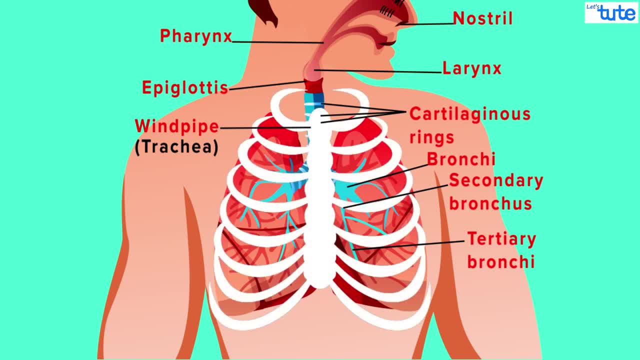 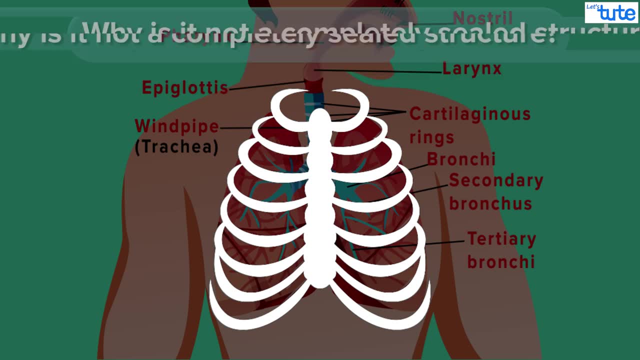 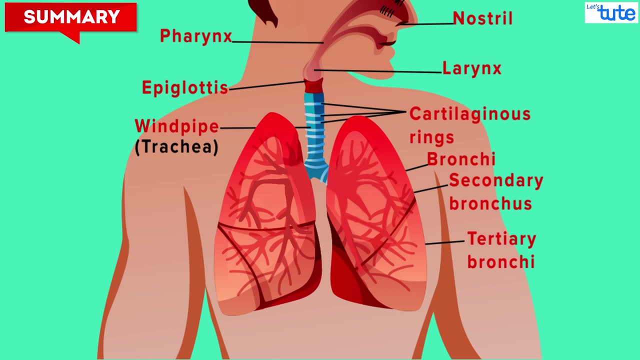 by a rib cage. Here is a question: Why does a rib cage have a cage like structure with gaps in between, and why is it not a closed, sealed structure? Think of it and share your response in the comment box below. So this was a session giving you a brief idea of the human respiratory system. It comprises. 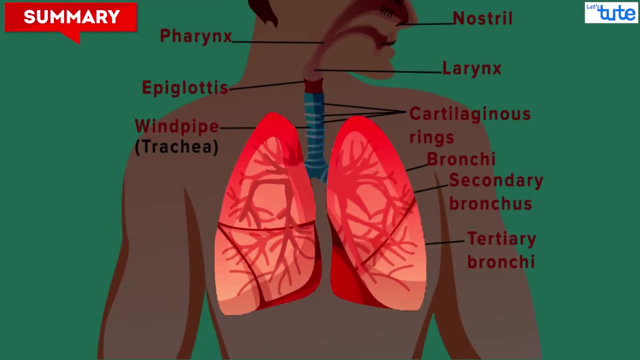 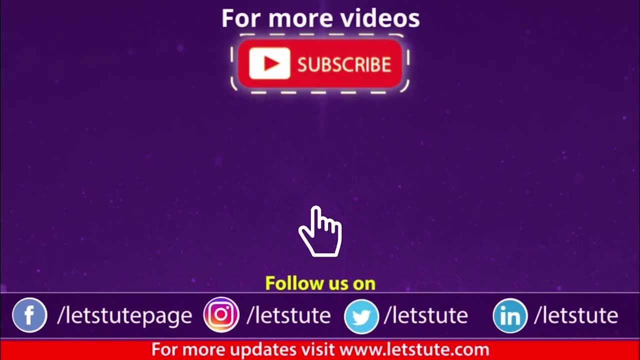 of the respiratory tract and lungs. In the next session, we will study about the mechanism of breathing. I hope you liked this session. If yes, then why wait? Hit that like button and subscribe to our channel for more such interesting science videos. Do not forget to press the bell icon. to receive updates from us. Thank you for watching.